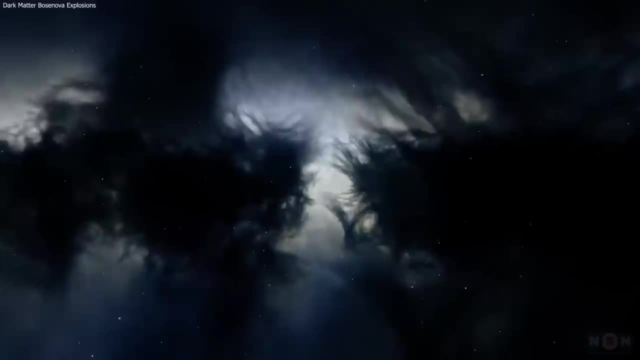 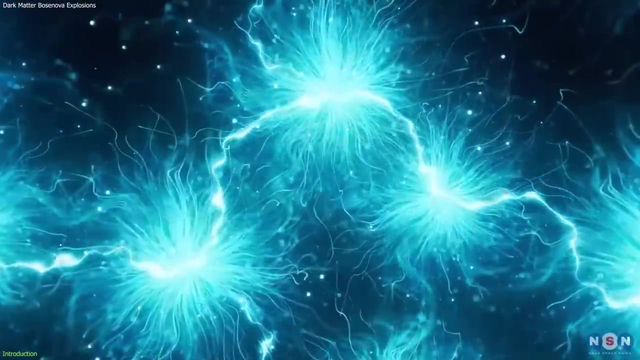 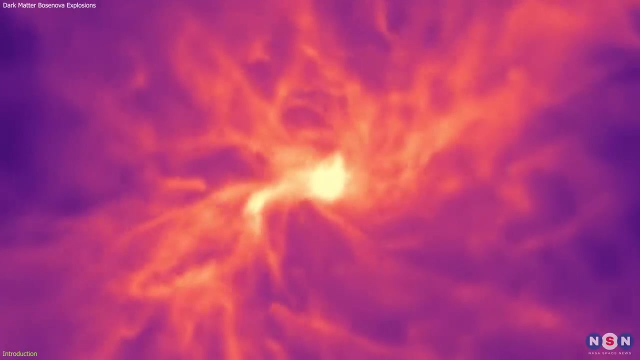 Dark matter is a ghostly substance that astronomers have failed to detect for decades, yet which we know has an enormous influence on normal matter in the universe, such as stars and galaxies. Through the massive gravitational pull it exerts on galaxies, it spins them up, gives them an extra push along their orbits or even rips them apart. 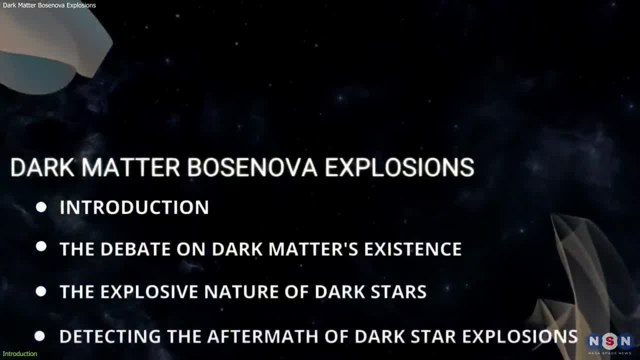 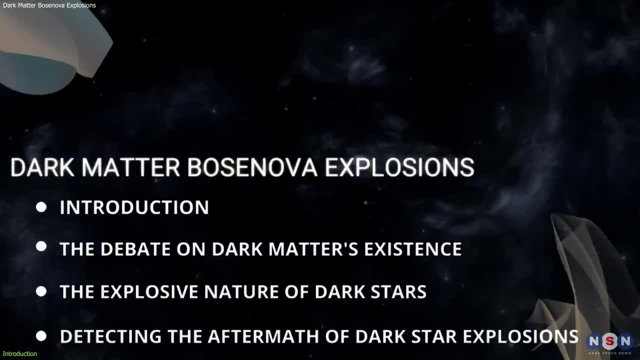 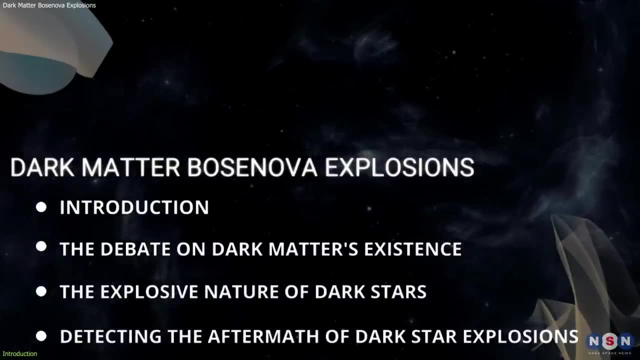 Today we dive into groundbreaking research that's challenging our ideas about dark matter and revealing the potential existence of dark stars. We'll explore the debate surrounding dark matter's existence, the explosive nature of dark stars and how detecting their aftermath could unveil the universe's secrets. 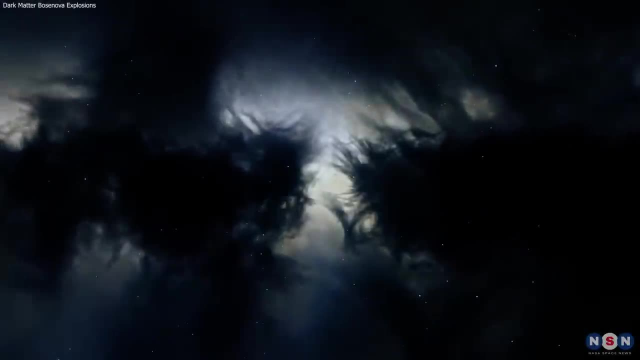 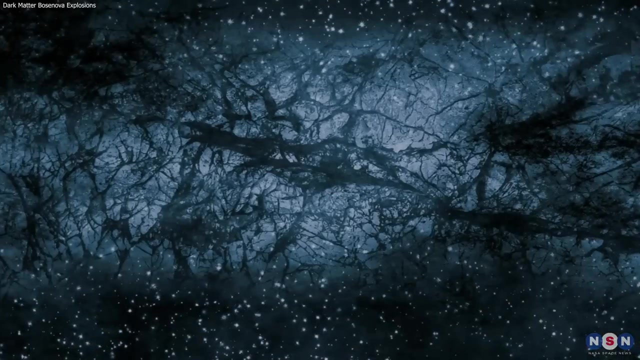 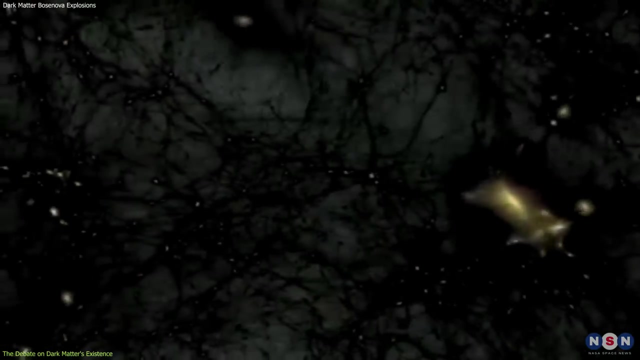 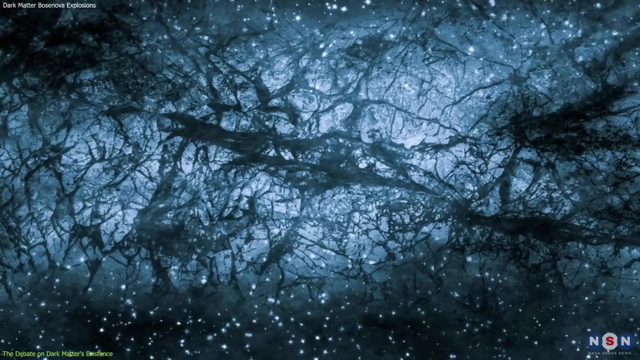 So, without further ado, let's unravel the mysteries of the dark universe together. The concept of dark matter has been a pillar of modern cosmology, shaping our understanding of the universe's structure and evolution. It's the invisible mass that holds galaxies together, yet its true nature remains one of the greatest mysteries in astrophysics. 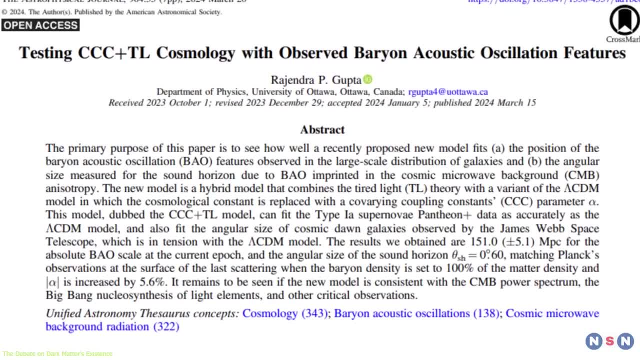 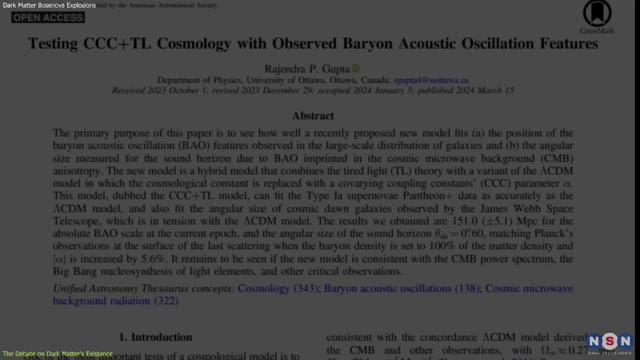 However, in a previous episode, we discussed recent research challenging the very existence of dark matter, proposing a universe that operates under different rules. At the forefront of this paradigm, SHIFT, is a study led by Professor Robert Kuhn, Professor Kuhn and Professor Rajendra Gupta from the University of Ottawa. 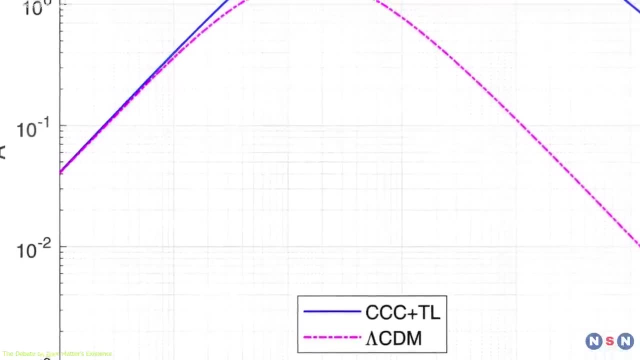 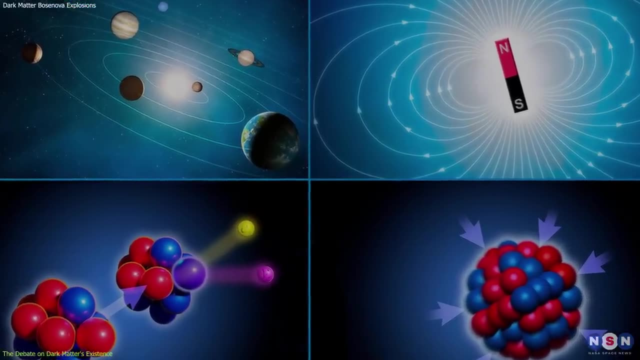 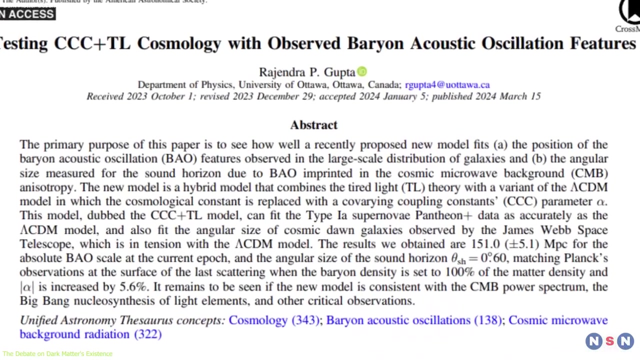 Gupta's research introduces the triple C plus tired light model. This model suggests that the forces of nature such as gravity and electromagnetism weaken over cosmic time and that light loses energy over vast distances. These ideas stand in stark contrast to the traditional view of a universe dominated by dark matter and dark energy. 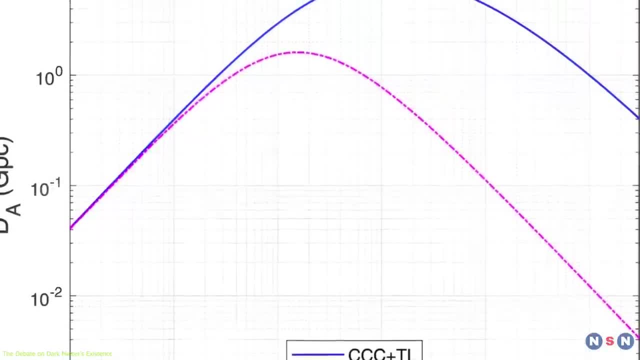 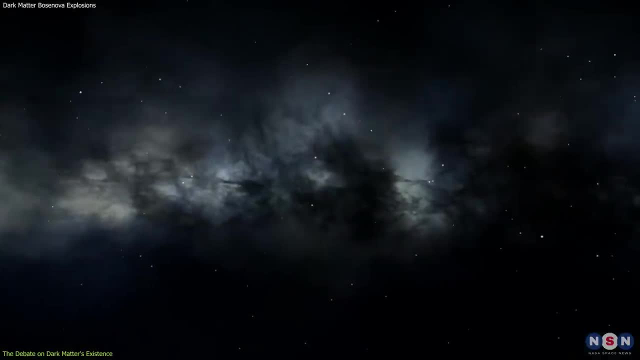 The combined model of triple C plus tired light challenges the conventional belief that dark matter may be the only source of light. The theory of dark matter makes up about 27% of the universe's mass, suggesting instead that the observed phenomena attributed to dark matter could be explained by the weakening of fundamental forces. 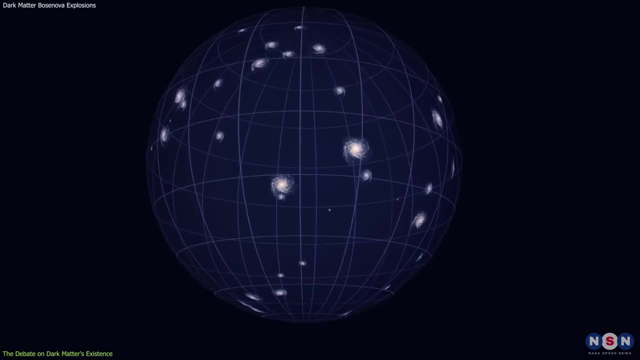 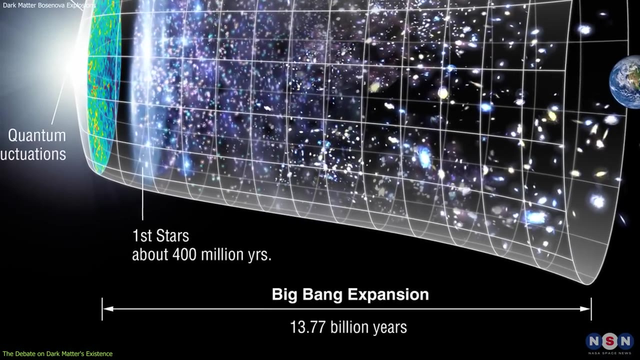 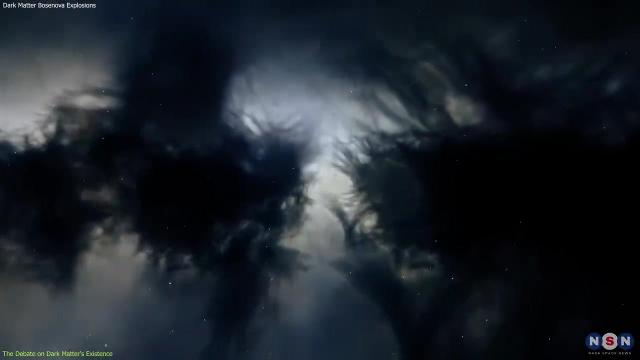 This theory also redefines the age and expansion of the universe, proposing that it is 27 billion years old, significantly older than the currently accepted age of approximately 13.8 billion years. If Gupta's model is accurate, it could mean that dark matter does not exist in the form we currently live in. This would challenge the necessity of dark matter's existence and suggest that the accelerated expansion of the universe is due to the weakening forces of nature, not the presence of dark energy. Moreover, this new model is consistent with various astronomical observations, including the distribution of galaxies and the evolution of light from the early universe. 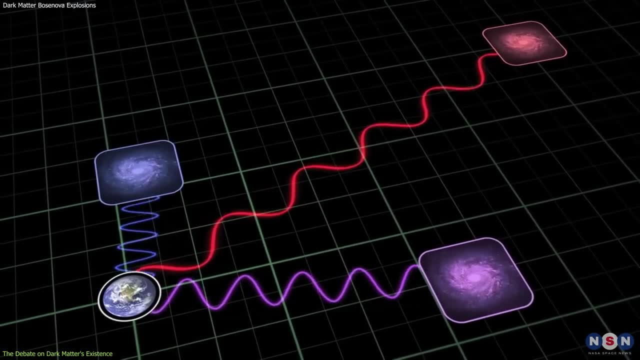 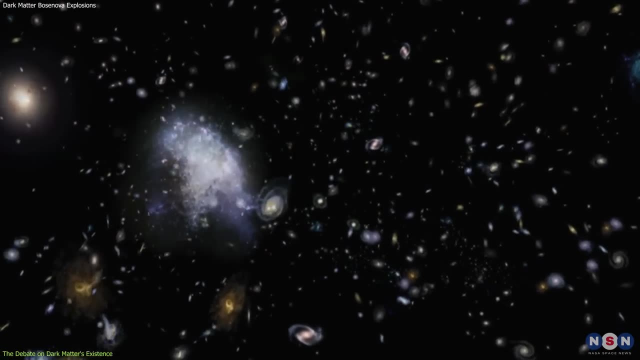 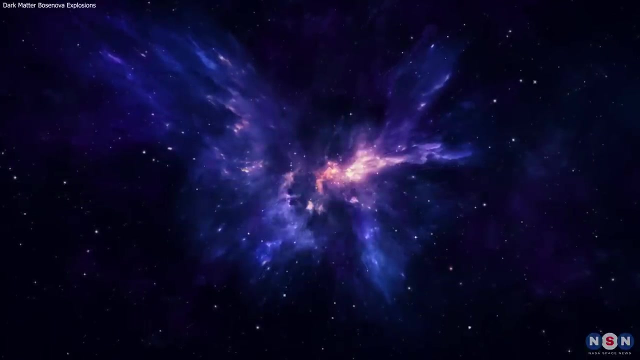 By analyzing redshifts and the angular size of the sound horizon, Gupta presents a compelling argument against the need for dark matter to exist. This research invites the scientific community to reconsider long-held beliefs about the cosmos and explore new avenues for understanding the fundamental forces and properties of the universe. 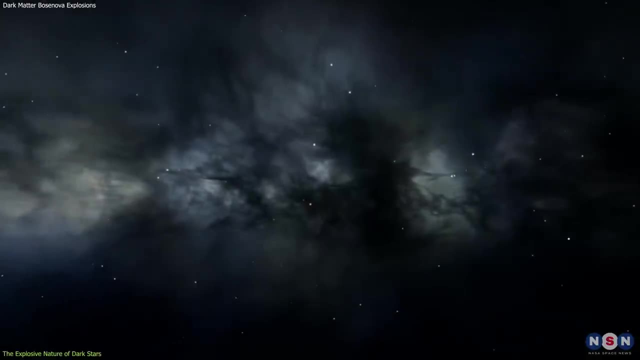 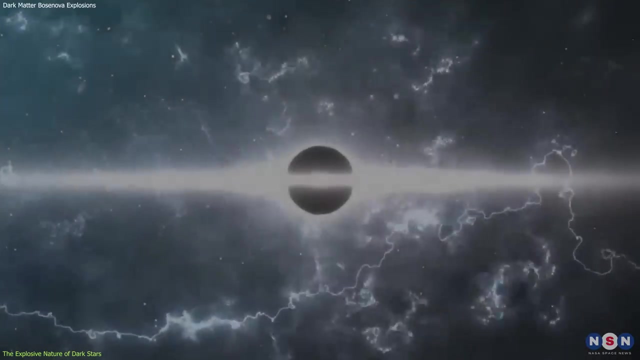 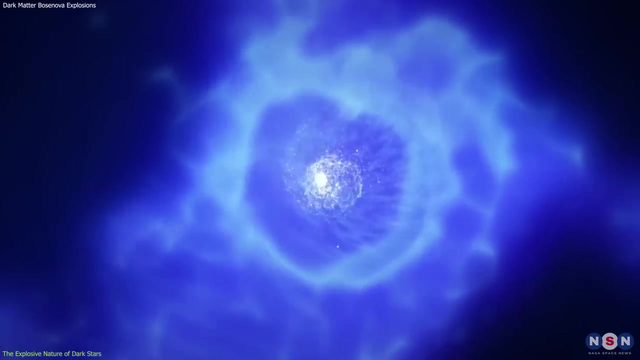 While the debate on dark matter's existence continues, there has been a fascinating development in theoretical astrophysics – the emergence of dark stars. These hypothetical stars, unlike their luminescence, are not necessarily stars. Unlike their luminous counterparts, are formed from dark matter particles, challenging our conventional notions of stellar formation and evolution. 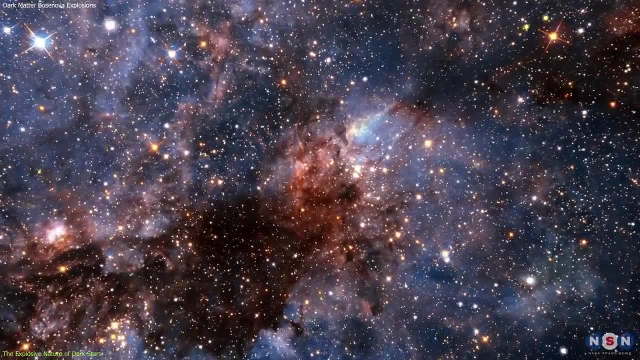 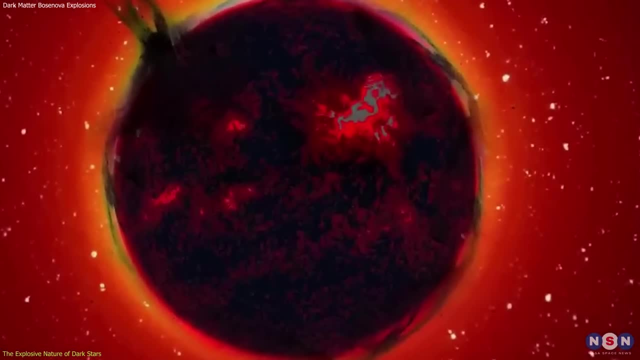 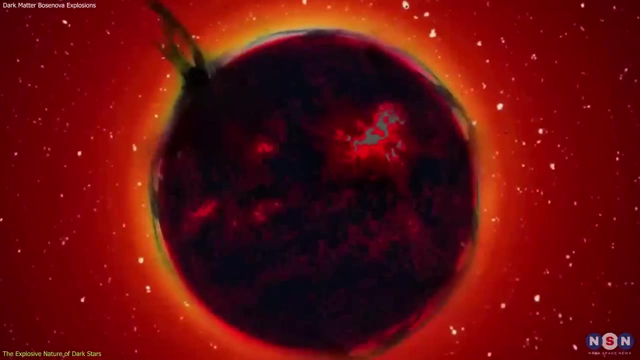 In the vast expanse of the cosmos where traditional stars have long been the celestial beacons guiding our understanding, dark stars propose a new paradigm where the enigmatic dark matter plays a central role in shaping the universe's structure and dynamics. At the heart of dark star theory are axions, a class of hypothetical particles. 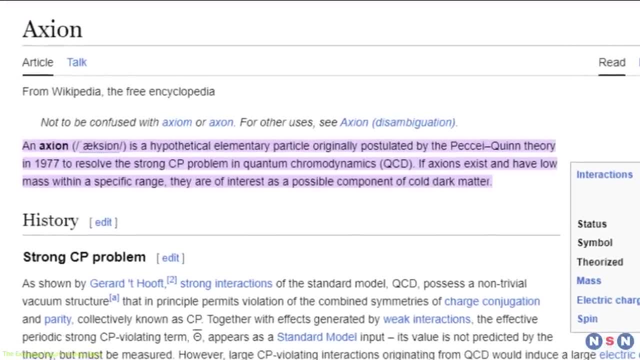 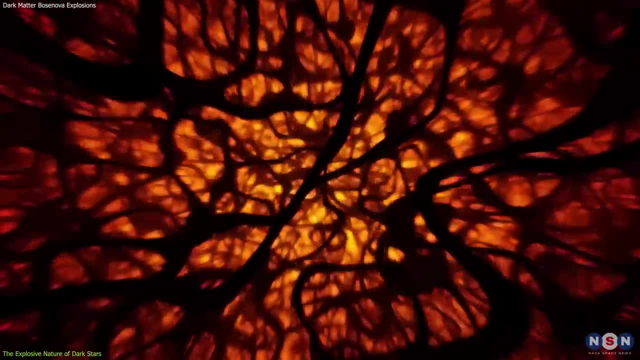 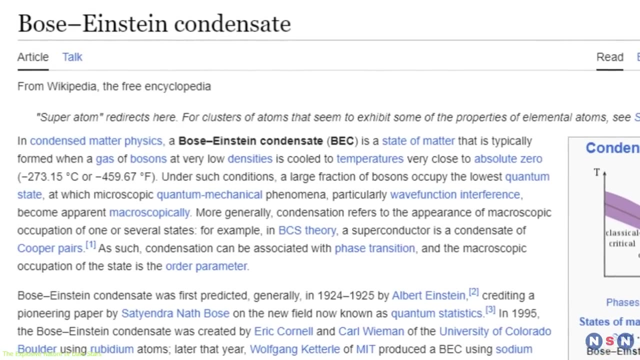 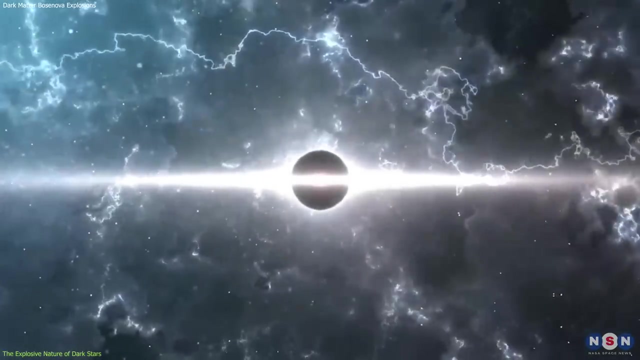 They are strong candidates for dark matter. Unlike WIMPs or weakly interacting massive particles, axions are incredibly light and can form Bose-Einstein condensates, a state of matter where particles behave collectively as a single quantum entity. This unique property allows axions to clump together, creating the conditions necessary for the formation of dark stars. 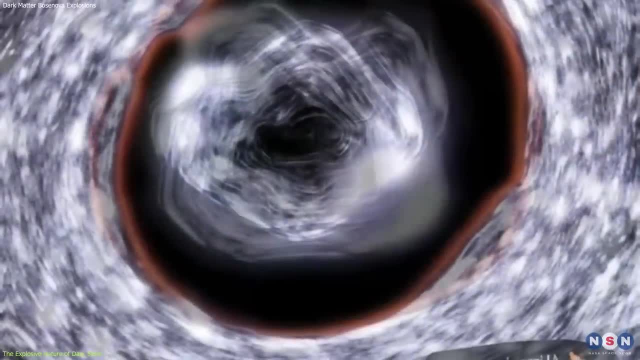 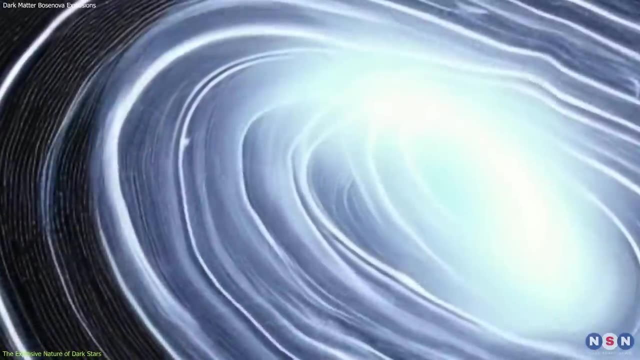 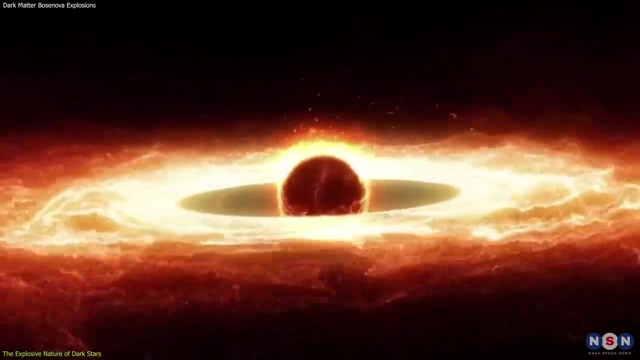 The formation of a dark star begins with a soliton, A localized lump of energy where axions are densely packed. As more axions accumulate, the soliton grows in size, eventually reaching the mass and size of a traditional star. However, dark stars are not stable entities. 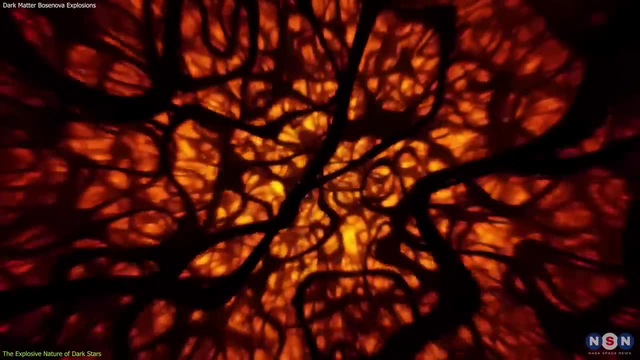 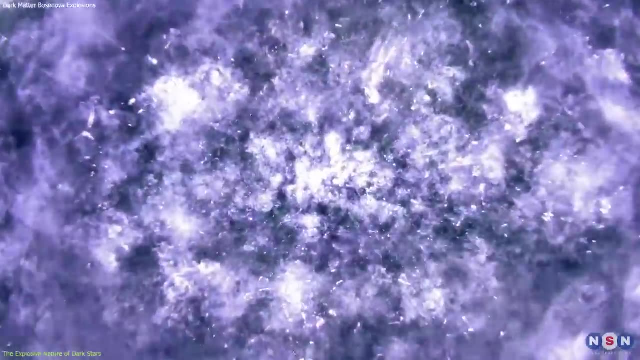 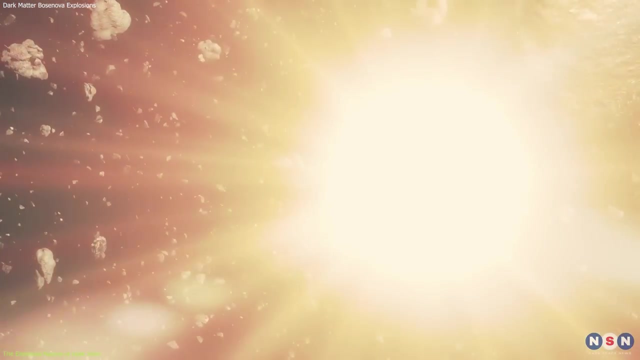 Their core, dominated by the Bose-Einstein condensate of axions, becomes increasingly unstable as it grows. This instability leads to a dramatic climax: The explosion of the dark star in an event known as a Bose-Einstein condensate, Releasing energy comparable to that of a supernova. 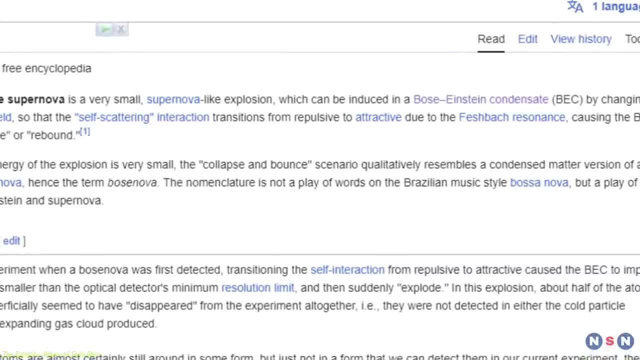 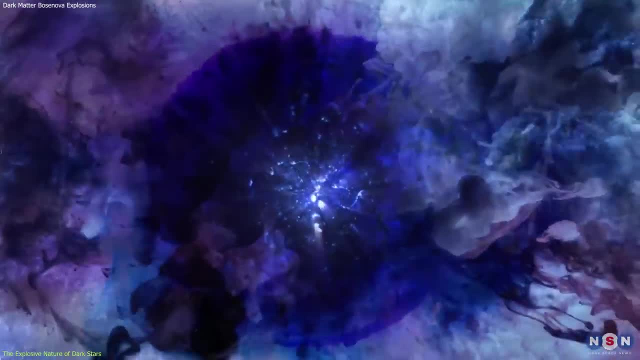 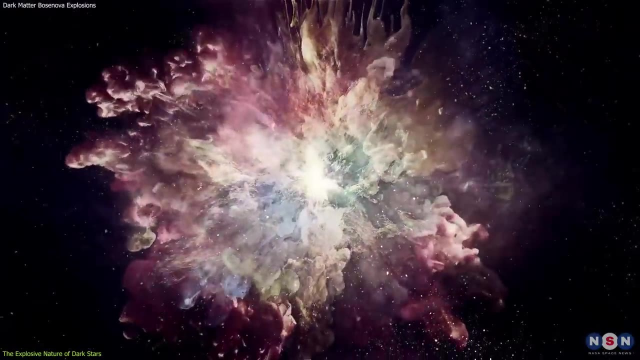 The concept of a Bose-Einstein condensate is derived from the term Bose-Einstein Nova, which refers to the explosive behavior of a Bose-Einstein condensate. When a dark star undergoes a Bose-Einstein condensate, it releases an immense amount of energy rivaling the most powerful explosions in the universe. 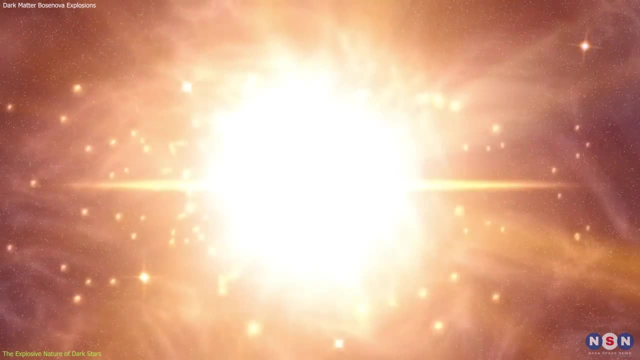 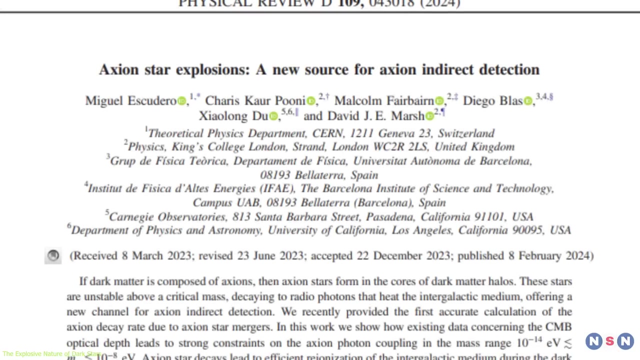 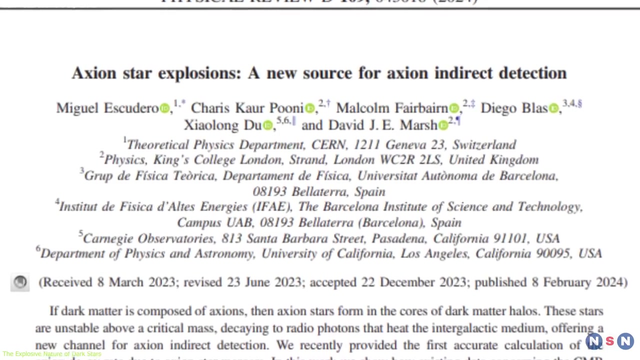 This event is not only a spectacular display of cosmic fireworks, but also a potential goldmine of information about the properties of dark matter. The study of dark stars and their explosive demise offers a unique opportunity to probe the elusive nature of dark matter, If axions are indeed responsible for these cosmic explosions. 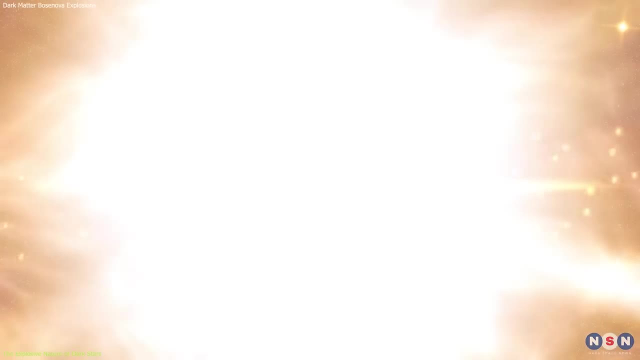 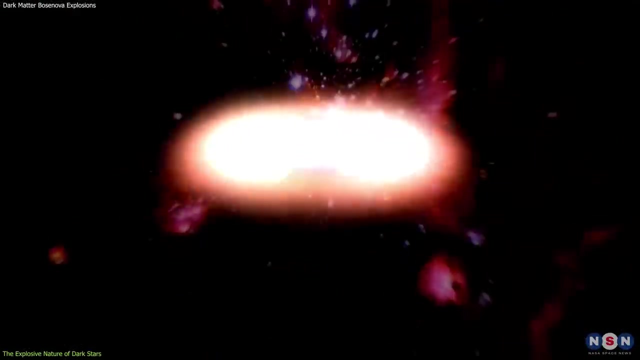 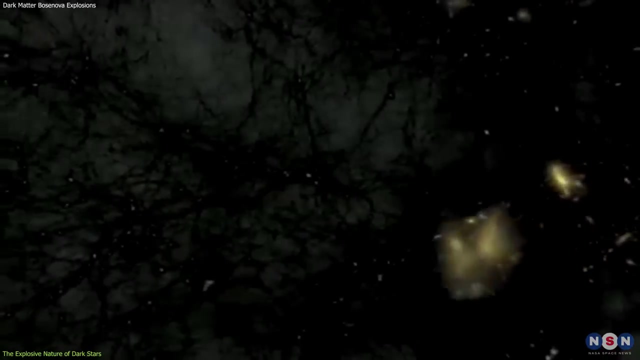 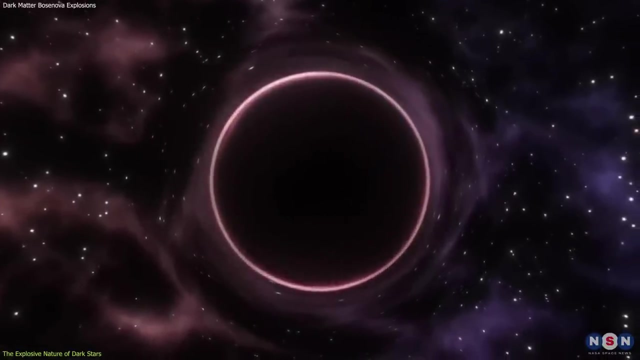 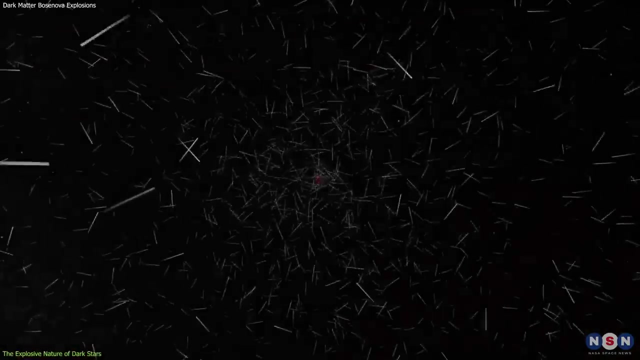 detecting the remnants of a Bose-Einstein condensate could provide direct evidence for the existence of these hypothetical particles. Furthermore, the energy released during a Bose-Einstein condensate could leave observable signs. The theoretical models of dark stars rely on assumptions about the properties of axions and their interactions, which are still poorly understood. 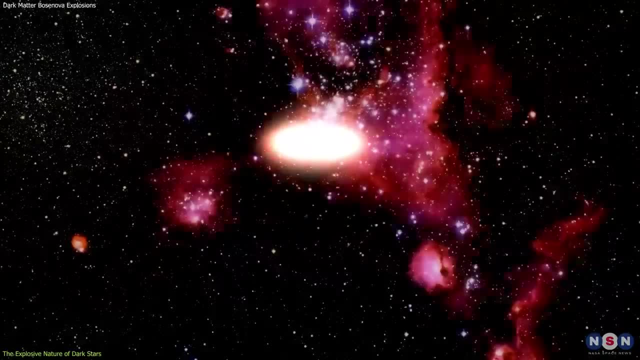 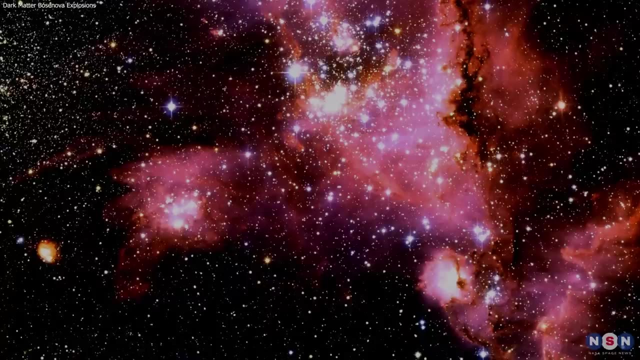 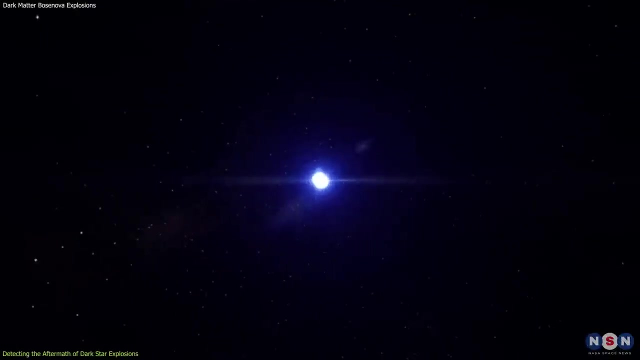 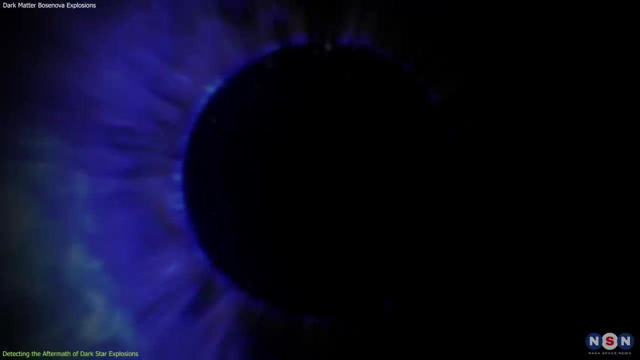 Additionally, detecting the aftermath of a Bose-Einstein condensate requires susceptible instruments capable of observing faint signals from distant regions of the universe. One promising avenue for detecting the aftermath of dark star explosions is through the observation of radio frequency emissions. When a Bossa Nova occurs, the energy released can ionize the surrounding hydrogen gas, causing it to emit radio waves. 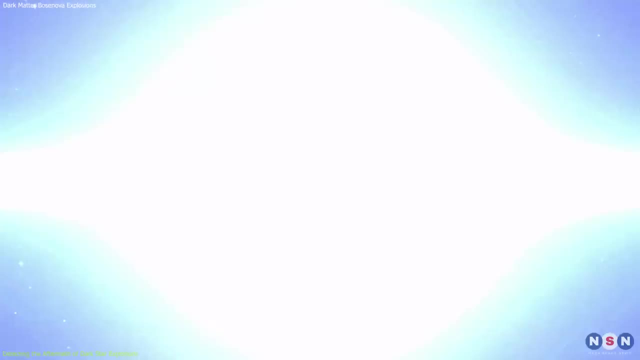 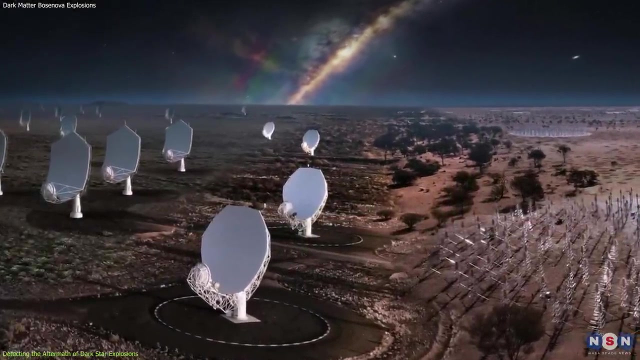 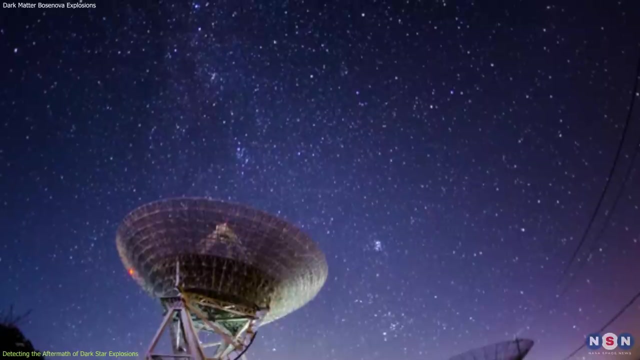 By analyzing these emissions, astronomers can infer the properties of the explosion and the nature of the explosion. By analyzing these emissions, astronomers can infer the properties of the explosion and the nature of the explosion. Advanced radio telescopes such as the Square Kilometer Array are poised to play a pivotal role in this endeavor, offering the sensitivity and resolution needed to detect these faint signals. 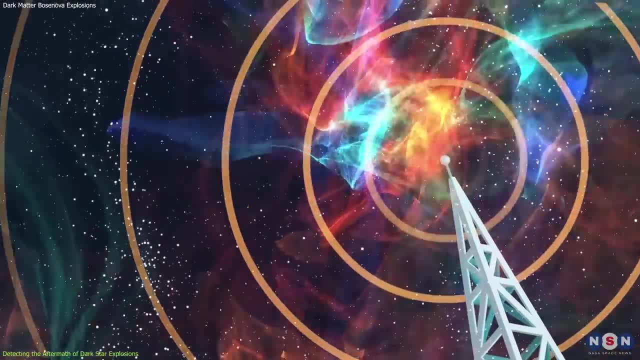 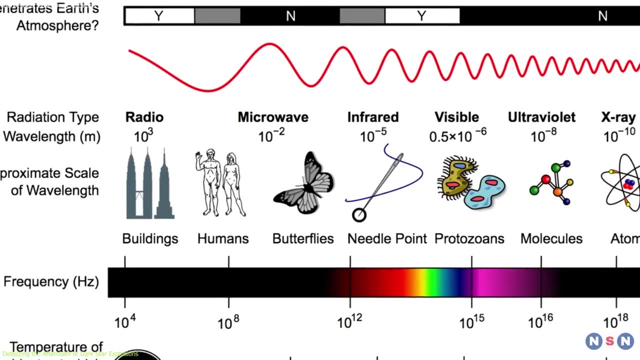 While radio observations are a key tool in detecting Bossa Nova remnants, a comprehensive understanding of dark star explosions requires a multi-wavelength approach. While radio observations are a key tool in detecting Bossa Nova remnants, a comprehensive understanding of dark star explosions requires a multi-wavelength approach. 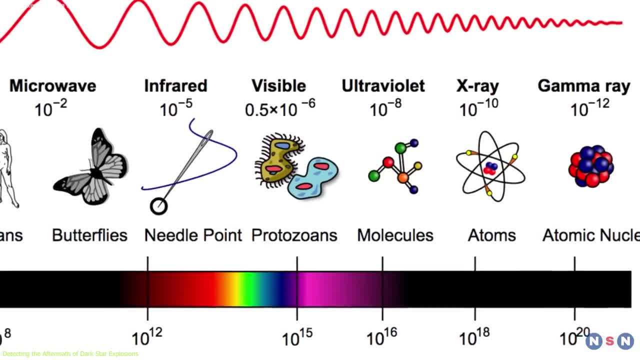 By analysing the particulars of those retroformal satu pientso instance of electromagnetic spectrum, such as X-rays and gamma rays, the ATL followed concentrate of帶子子子 can provide complementary information about the energy and dynamics of the explosion. 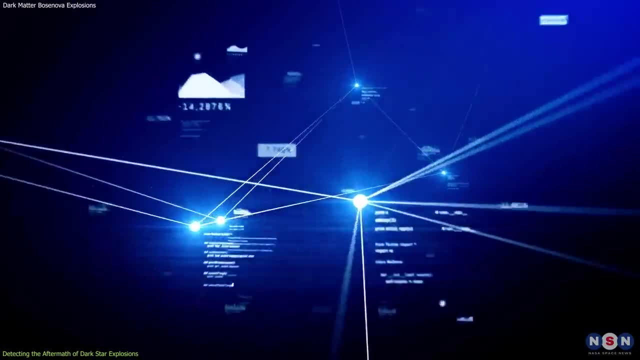 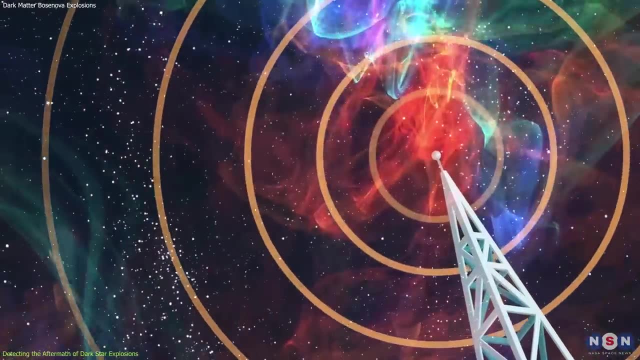 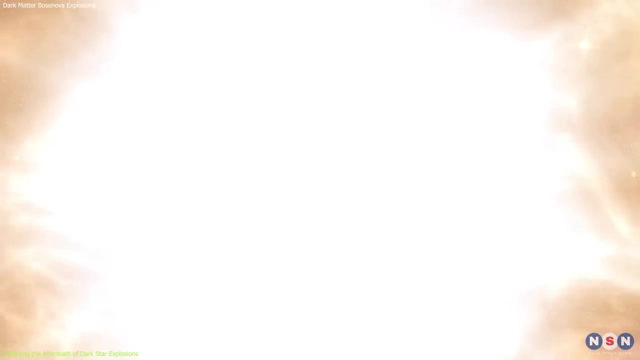 Combining data from different wavelengths will help build a more complete picture of these enigmatic events. Despite the potential for ground-breaking discoveries, detecting the remnants of the dark star explosions is a challenging task. The signals from these events are expected to be faint and could be easily obscured by other sources of cosmic radiation.